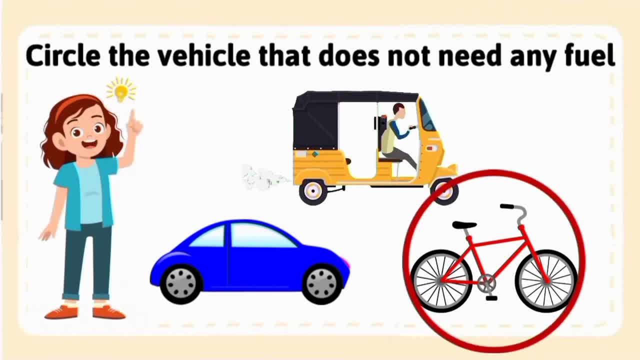 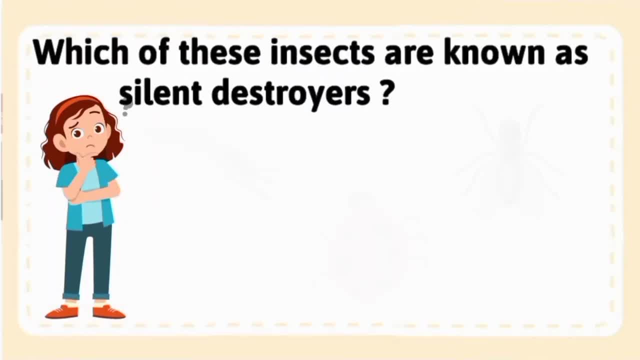 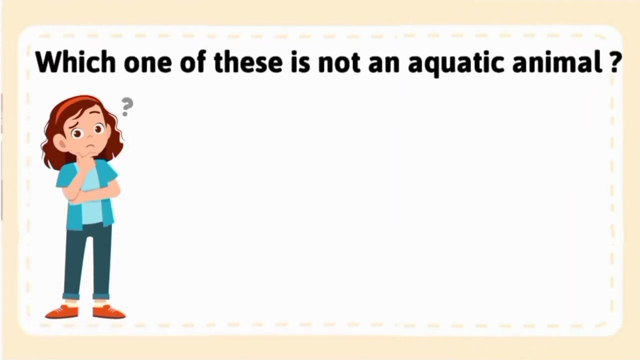 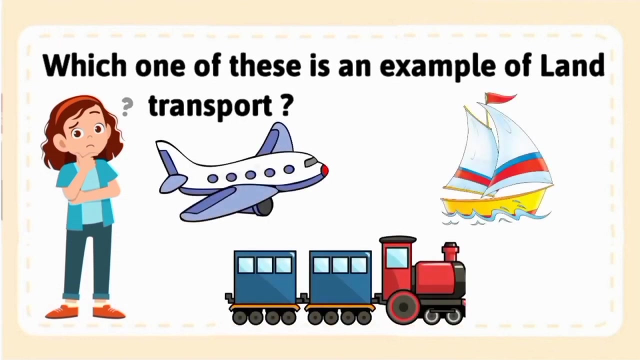 It is the bicycle. Which of these insects are known as silent destroyers? The correct answer is termite. Which one of these is not an aquatic animal? The answer is rat. Rat is not an aquatic animal. Which one of these is an example of land transport? 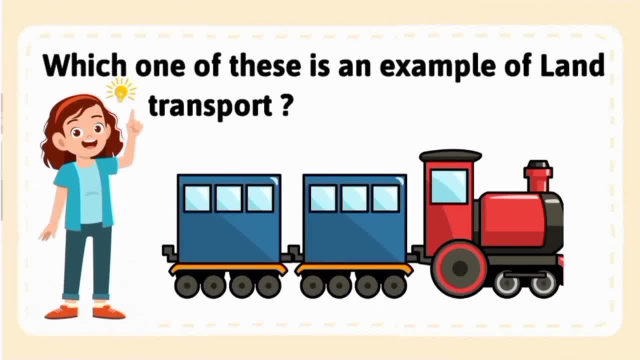 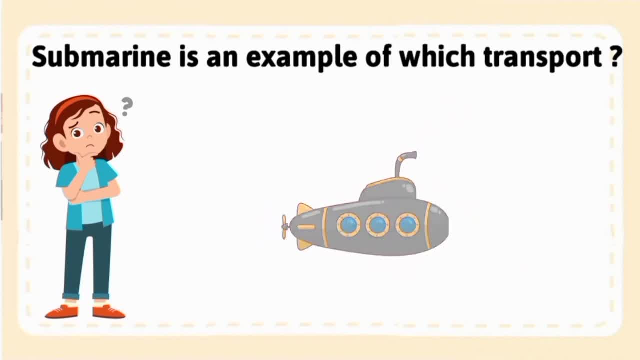 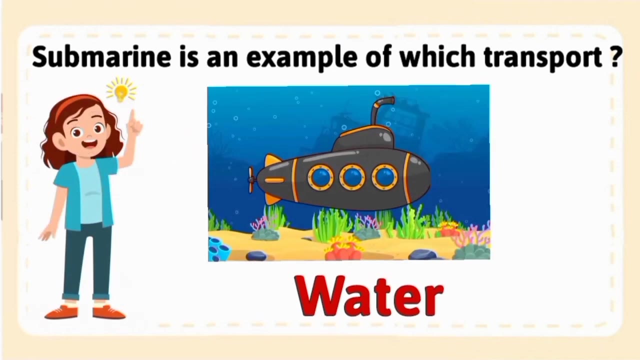 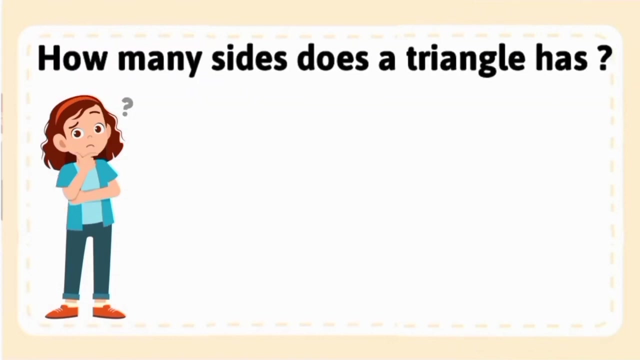 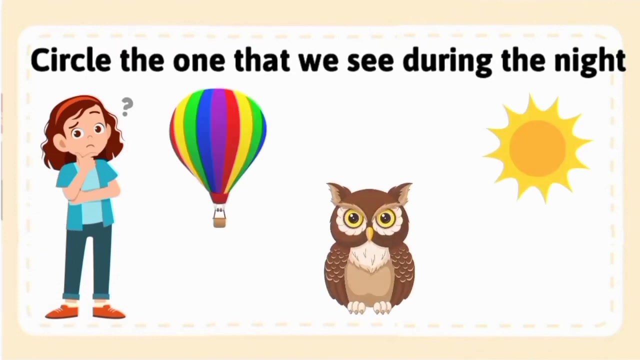 It is the train. Submarine is an example of which transport. Submarine is a water transport. How many sides does a triangle has? A triangle has three sides: Circle, the one that we see during the night. Circle, the one that we see during the night. 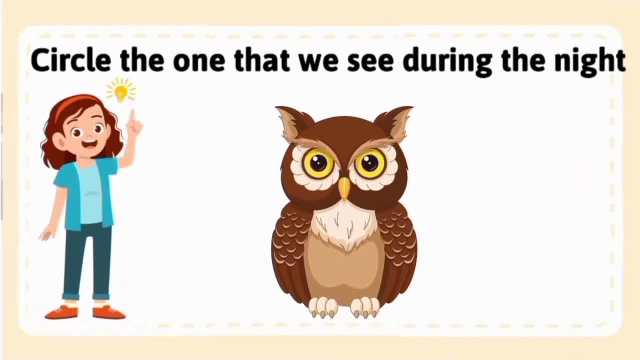 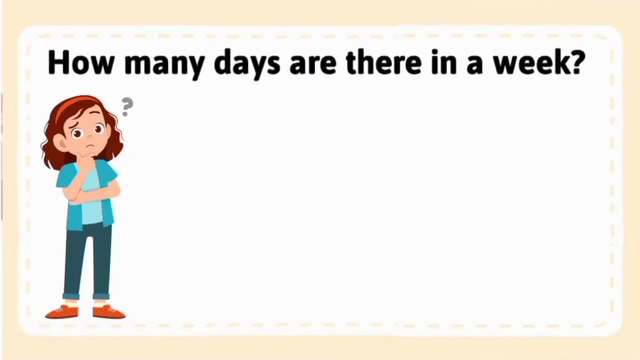 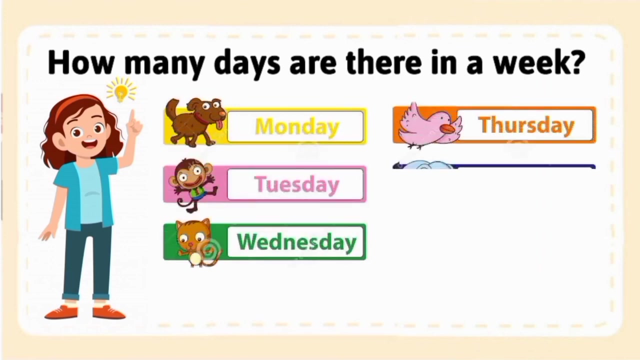 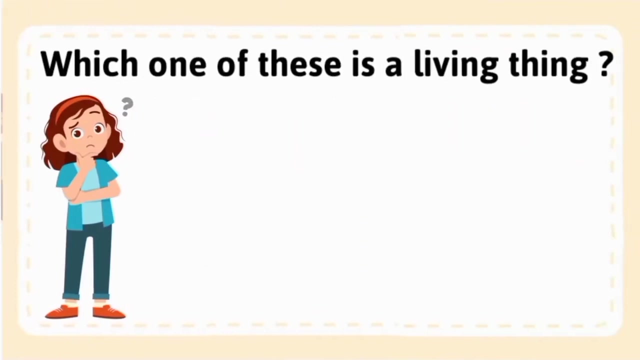 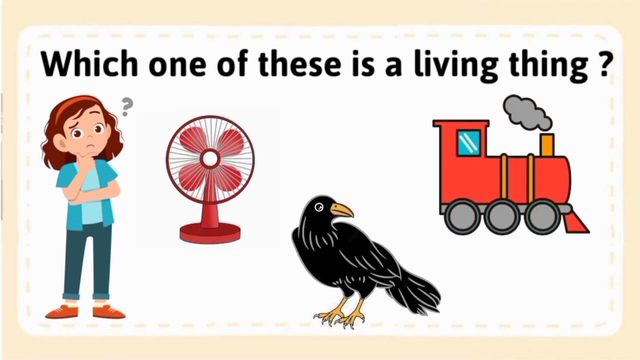 We can see an owl during the night time. How many days are there in a week? There are seven days in one week, and they are Monday, Tuesday, Wednesday, Thursday, Friday, Saturday and Sunday. Which one of these is a living thing? 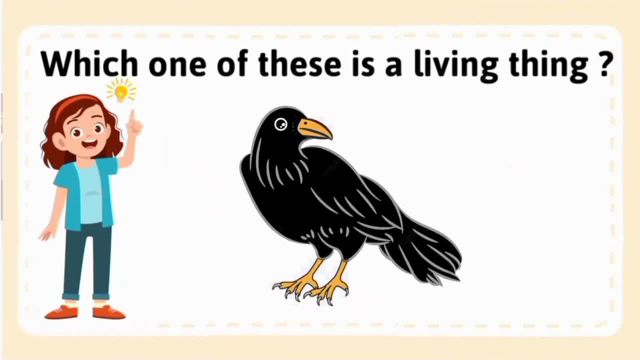 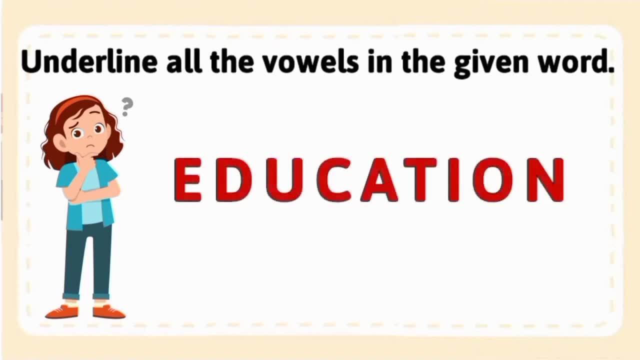 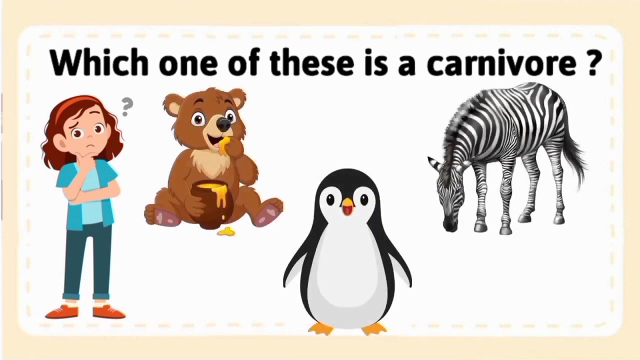 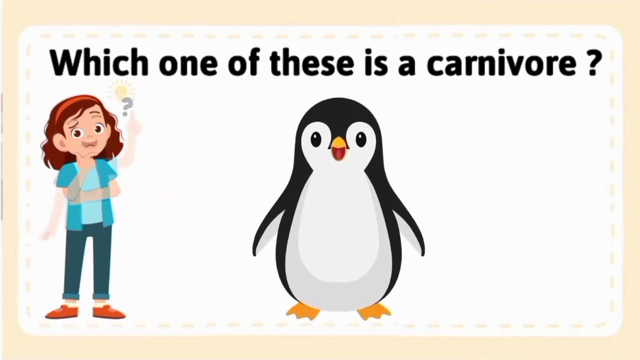 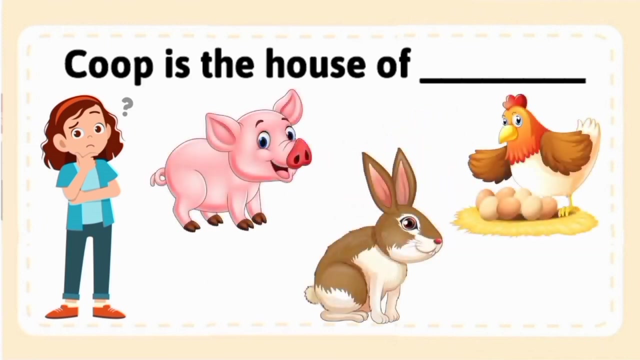 A crow is a living thing. Underline all the vowels in the given word. Which one of these insects are known as silent destroyers? Which one of these is a carnivore animal? The correct answer is penguin. Coop is the house of which animal? 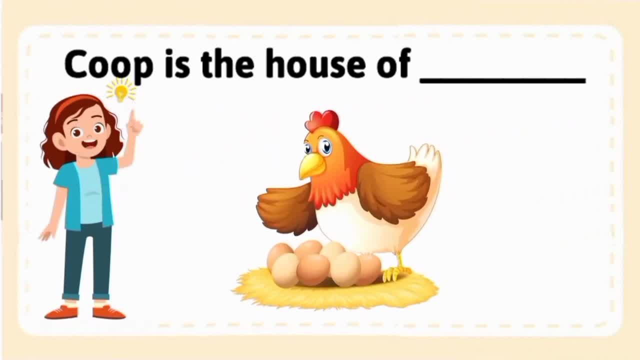 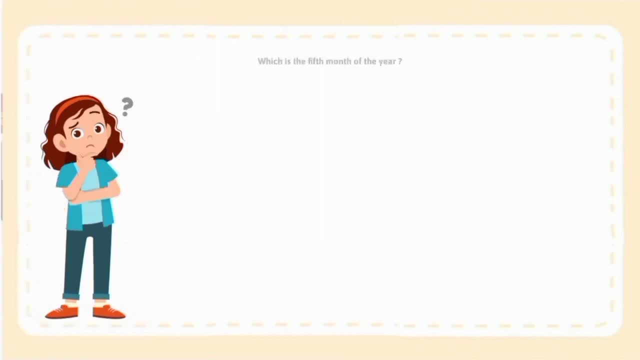 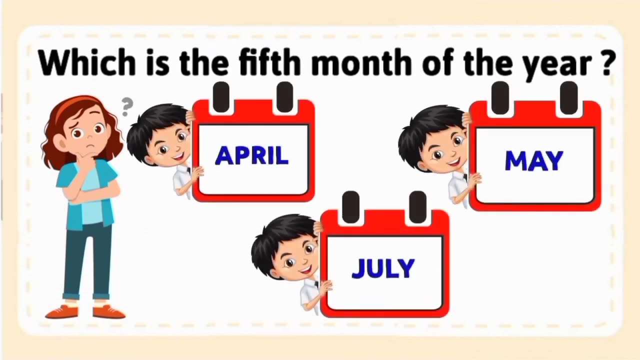 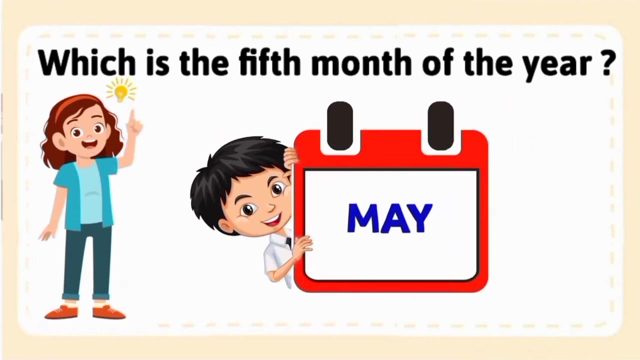 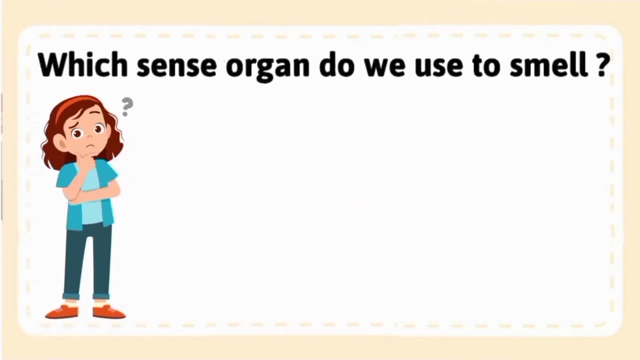 The correct answer is hen. Hen lives in a coop, Which is the fifth month of the year. May is the fifth month of the year. May is the fifth month of the year. Which sense organ do we use to smell? It's the nose. 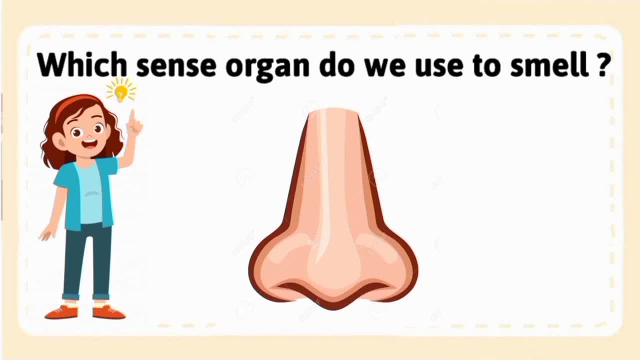 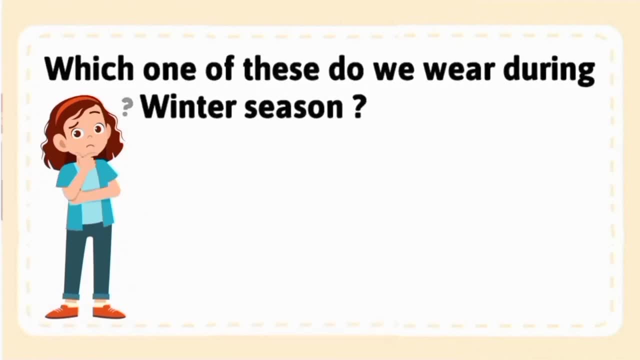 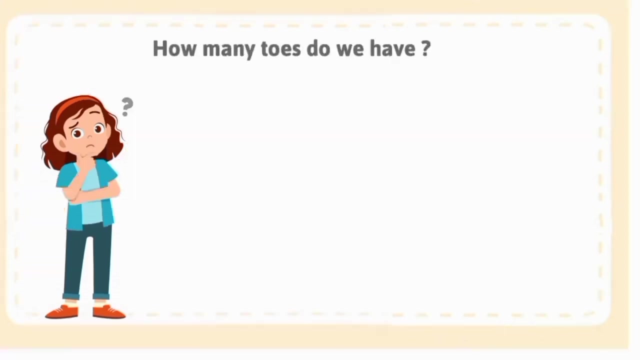 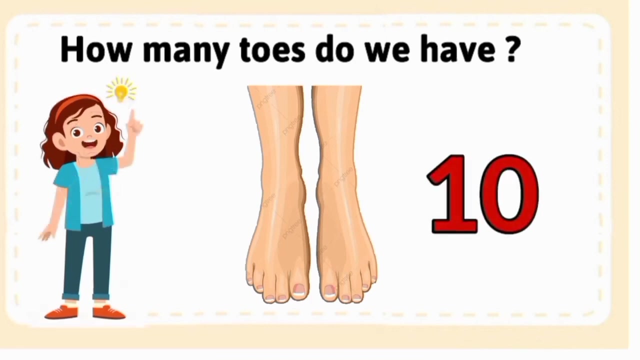 We use our nose to smell different odours around us. Which one of these do we wear during the winter season? Mittens. We wear woolen mittens to keep our hands warm. How many toes do we have? We have ten toes. 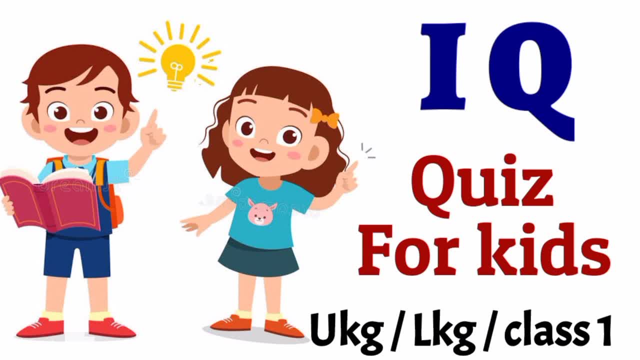 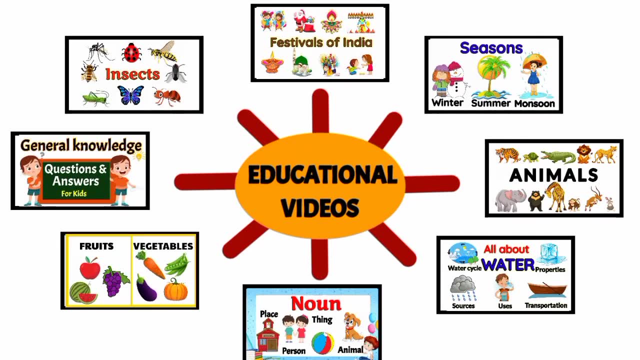 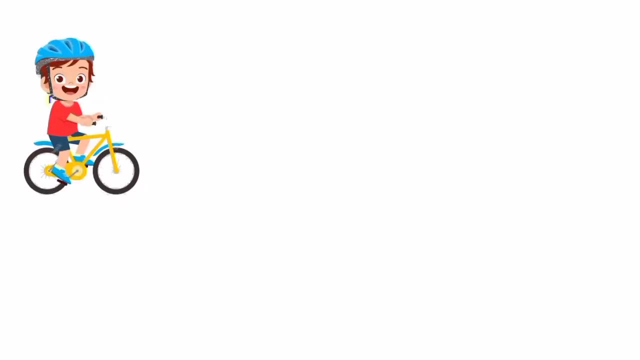 Let's feed our teeth. Great game, Great. God bless you. Cheers, Cheers guys, Cheers, Cheers, Cheers guys, Cheers great Cheers guys, Cheers you.